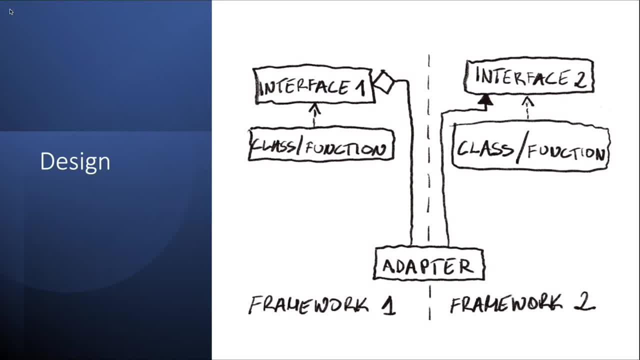 instances of objects that implement it. And in between, there on top of the dotted line, you see the adapter, And so adapter here will adopt something from framework one so that it can be consumed by framework two, And it does so by implementing the interface from framework two and holding a reference to. 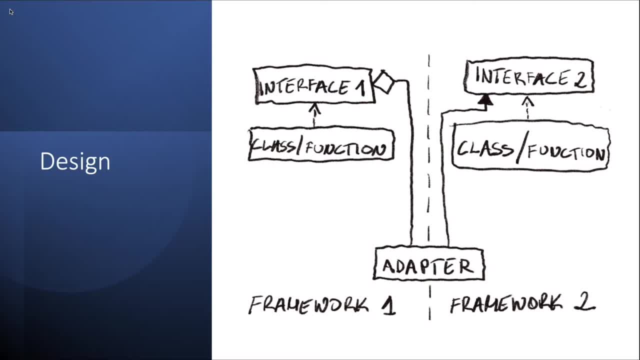 something from framework one. So then instances of the adapter can be passed to classes or functions that would normally only accept interface two, And this adapter implements that interface and whatever call it receives, it will be able to implement it. And then on the right, you see the. 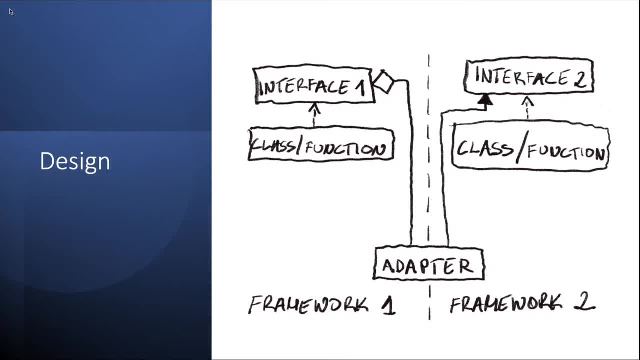 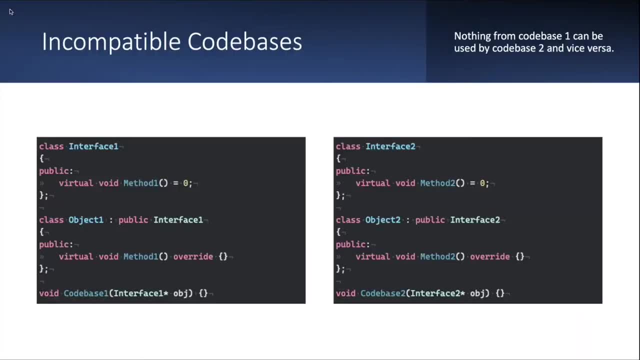 interface that have this interface one And we will implore that user to, if it receives on that interface, it will translate it accordingly to fit into interface one. So here's the implementation of two incompatible code bases And if you look at the left you have your interface one object. 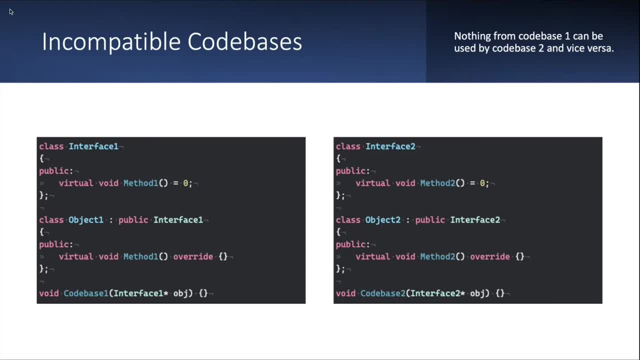 one that implements this interface, that has a method one and some code base, one function that operates on an instance of this, of these objects or these interfaces- Brookabae And over here one more same case: interface 2, method 2, object 2, code base 2 and, as it is, these code bases are incompatible. 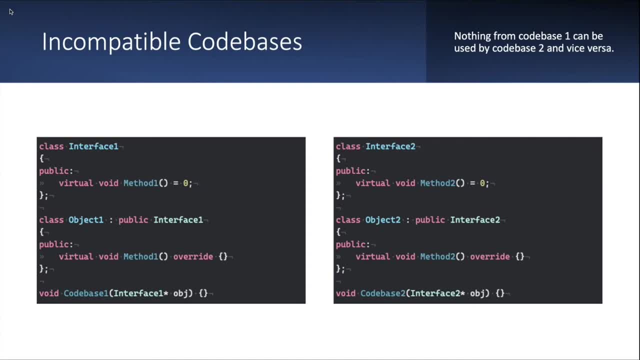 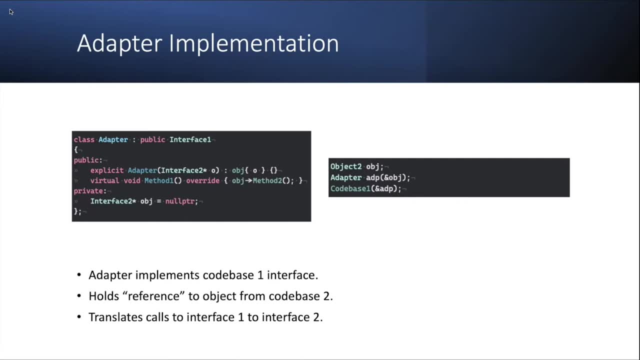 so nothing from code base 1 can be used by code base 2 and vice versa. so here's the implementation, simple implementation of the adapter itself. so you'll see that on the left you'll see the implementation of the adapter. it implements the interface 1 and then, when it is constructed, it 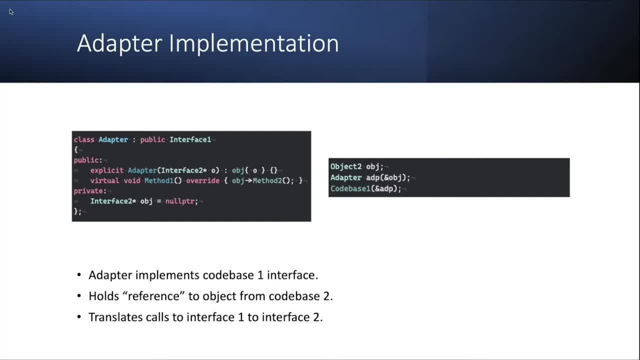 takes a pointer to some instance of interface 2 and finally you'll see that it implements the method 1 from interface 1 and in this example it merely does a call on the method 2 from interface 2. but a more more complex example could change parameter types. maybe do some tweaking to the 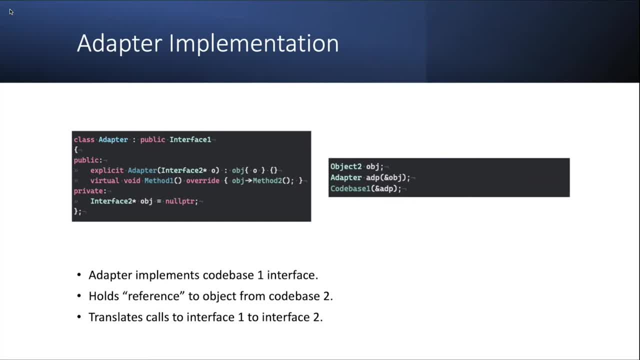 parameters, accept different number of parameters and pass some dummy parameters or or create some some values, if if the parameters to these methods were were different. so this is also an example of a non-owning adapter. it only holds a pointer. it's not responsible for the lifetime. 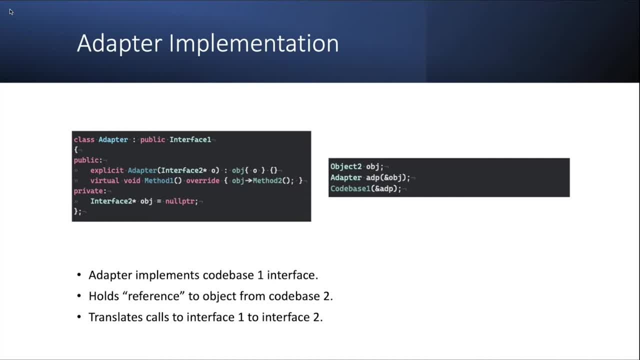 of the object it points to, but this could easily be changed. it could you know, hold, hold something some object to that implements interface 2 by value, or if only have a unique pointer to it, and that it would be responsible for its lifetime. and on the right, you will see that now i'm able to. 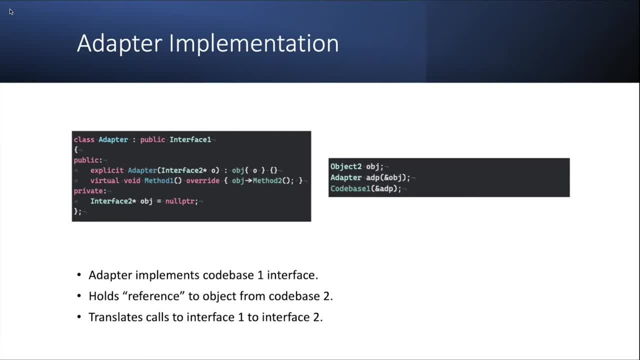 create an instance of object 2, pass an address of it to the adapter and then pass the adapter to code base 1, and the adapter is responsible for translating these calls, and code base 1 is completely unaware that it's now using some object from completely different code base. this could be: 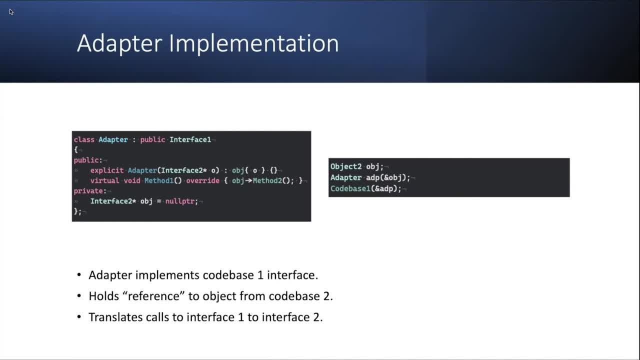 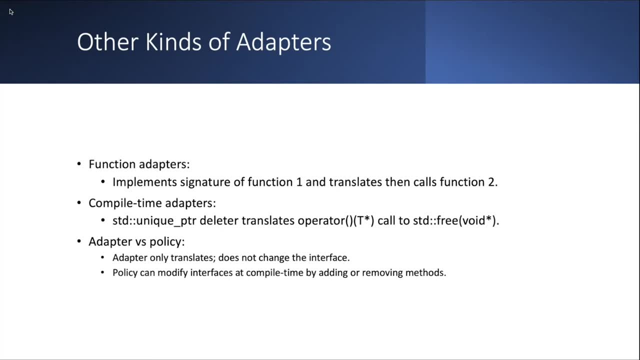 a library or a file, whatever module, anything right. author also talks about different kinds of adapters, to name a few, or function adapters. so that's, that's very simple idea. you have a, you have something that accepts a function with a given signature and you create the function with that. 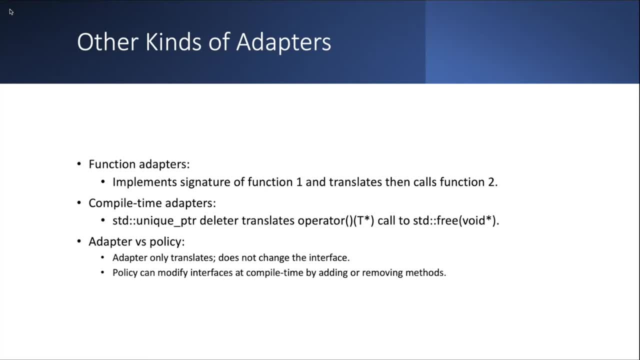 signature and then translate whatever parameters are given to you during the function. call to the signature function too. um, there are compile time adapters. an example would be something like a deleter from- uh, from unique pointer. a unique pointer expects an instance of something that is a functor. so 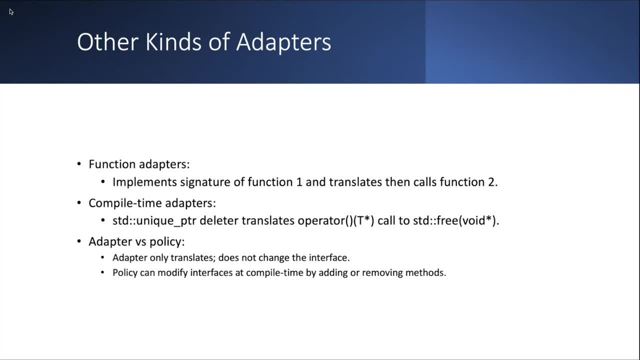 some object that implements the function call operator and said adapter can implement this, this function operator, and, for example, translate it to to a call to std3. um, finally, author talks about adapter versus policy and i don't think they're really related at all, but well, it's mentioned there, so i'll mention it also. adapter's job is really only to translate. 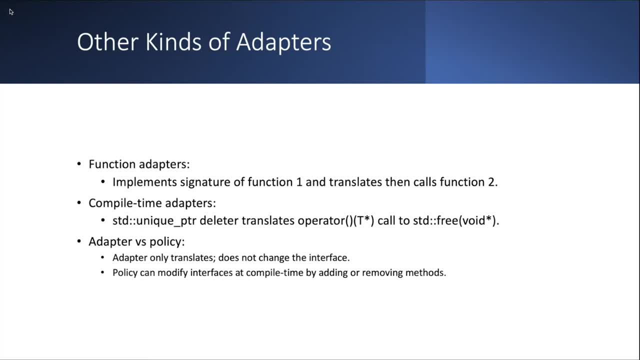 from one interface to the other, not decorate the interface, not change any of it, just simply make, make the translation between two incompatible interfaces, whereas a policy- as as we discussed a few weeks ago, you know, a policy can- can change the interface or decorate it, can add to it or